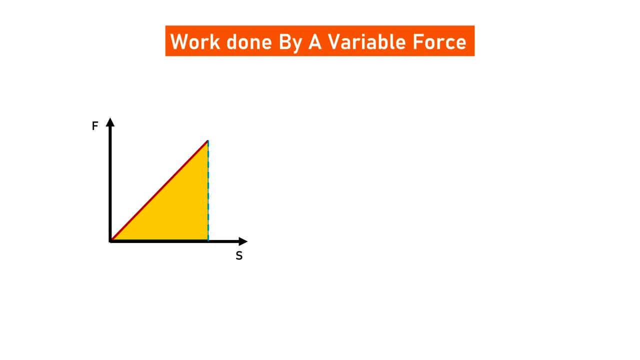 of the triangle formula. Here, the height of the triangle will give the force applied and the base of the triangle will give the displacement. Let's apply the area of the triangle formula- The area of a triangle is equal to half of the base- into. 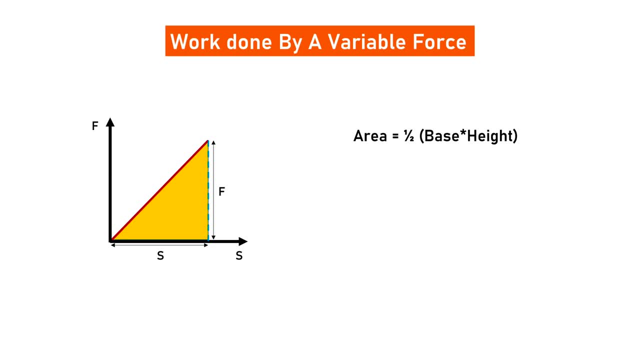 height. Just substitute the value of height and base and we will get area is equal to half of S into F. Rearranging this equation, we will get half into F, s, N 2's. Here you can observe that on the right-hand side we are getting the product of force. 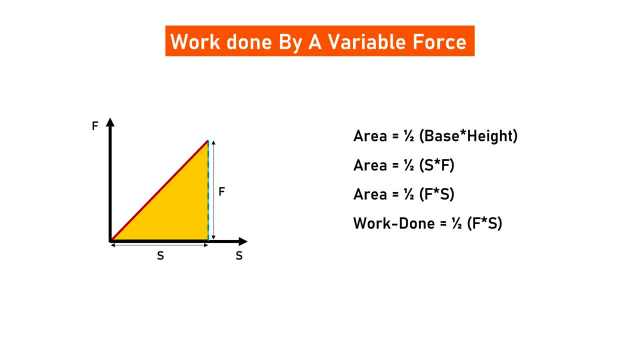 and displacement. It means that we are indirectly getting the work done. From this we can say that area under force and displacement will give the work done by the variable force. Now let us consider a graph between force and displacement and you can observe that the force is variable In this case. to find out, 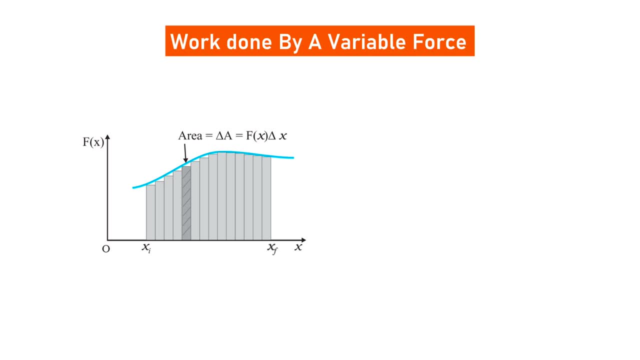 the area under the graph. we can divide the area into small rectangular pieces. In that, consider a rectangular strip. If you take this side of the rectangle, you will get the value of force, that is, f of x. and if you take this side of the rectangle, then you 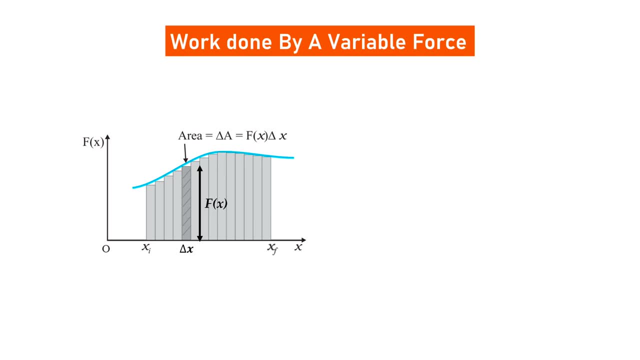 will get the small displacement that is delta x. Now just find the area of this rectangular strip that is delta- a is equal to f of x- into delta x. Here you can observe that on the right-hand side we have the product of force and displacement. It means that we are 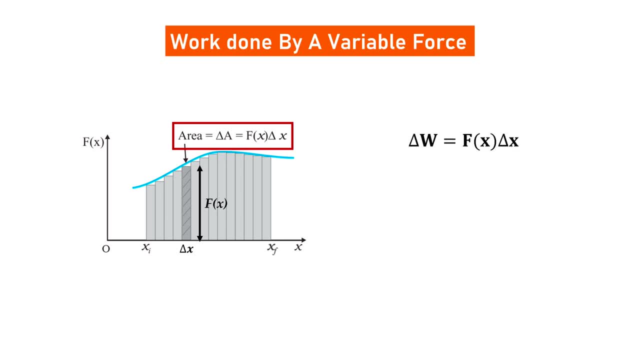 getting the small work done for a small area. Now to calculate the total work done: from the initial point x is equal to f of x. we have the product of force and displacement From the initial point xi to the final point xf. we just need to integrate between the. 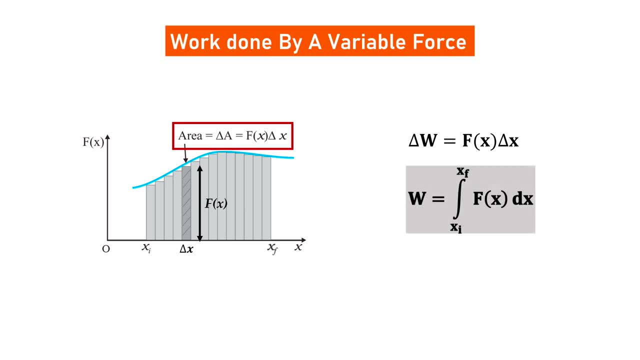 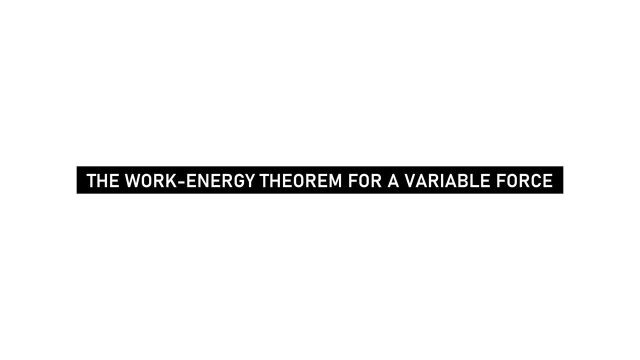 limits xi and xe. That is how we calculate the work done for the variable force. In the next video I will be explaining the work. Energy Theorem for a Variable Force. Thank you. 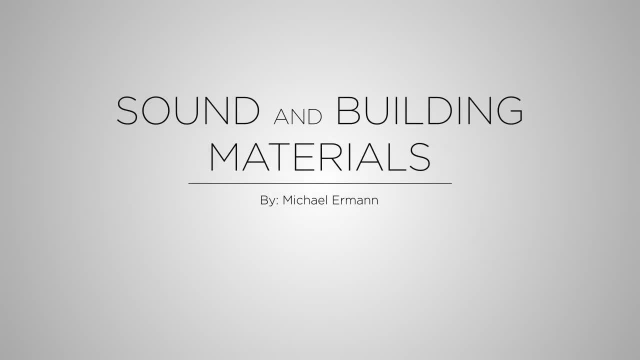 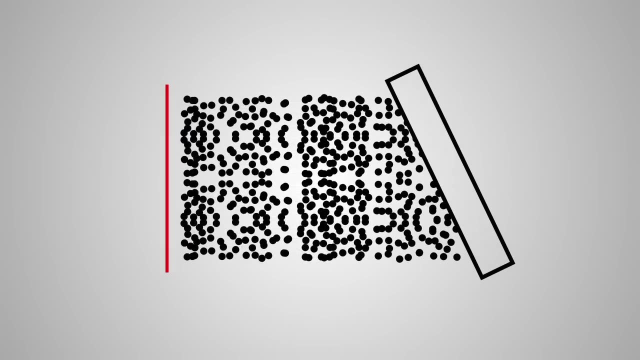 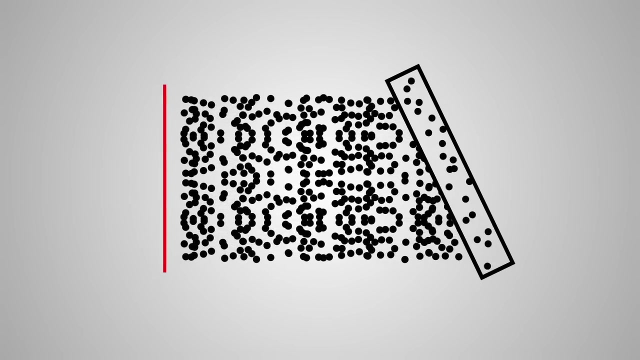 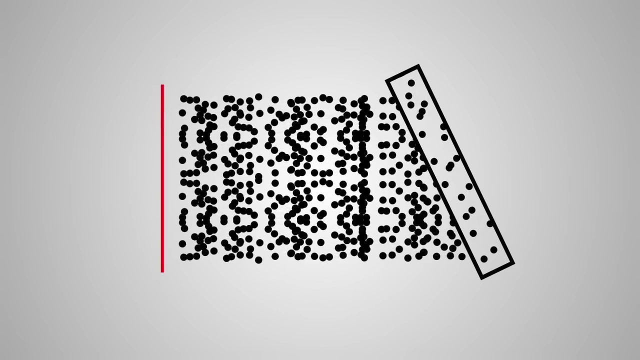 When sound impinges on a surface like that found on a building's interior, some of the energy passes through. Some of the sound energy is absorbed and reassigned as heat within the material. You can't make the wall hot by yelling at it. It's not that much heat.